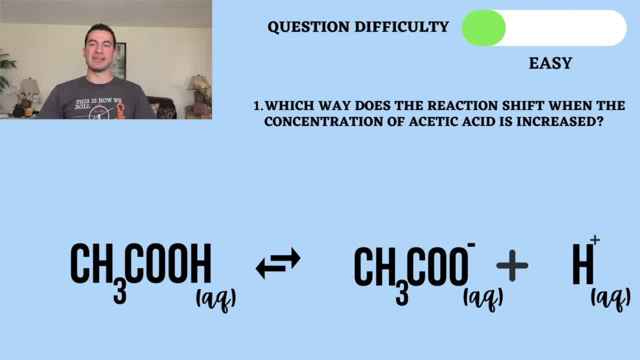 So for question one, we're presented with the acid dissociation of acetic acid. And if you guys don't know what acetic acid is, think about vinegar, because acetic acid is found within vinegar. So we're presented with this question. 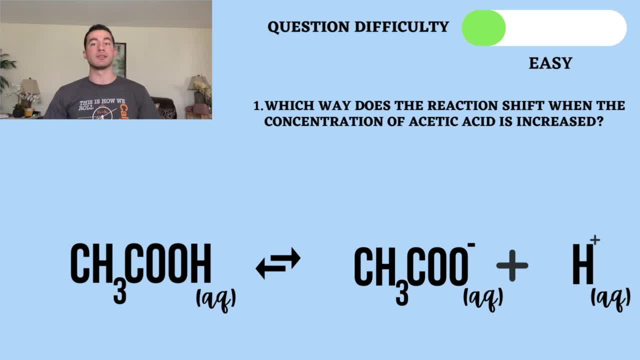 in which we have acetic acid dissociating into its ionic form and its conjugate base. So which way is it dissociating? Does the reaction shift when the concentration of acetic acid is increased? Well, if you increase the concentration of acetic acid, 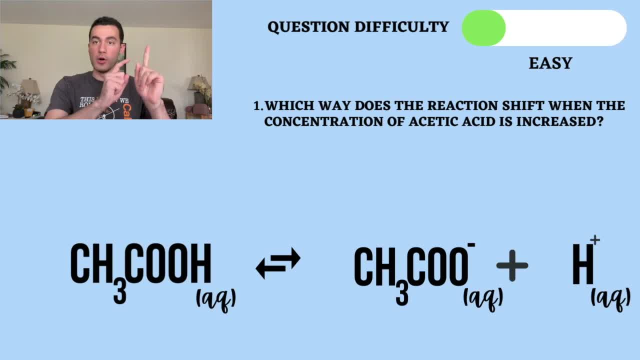 you're increasing the concentration of the reactants, So the equilibrium is going to shift right in such a way that it's going to relieve the stress from the excess reactant and put the stress on the products, since we have more reactant than we do products. 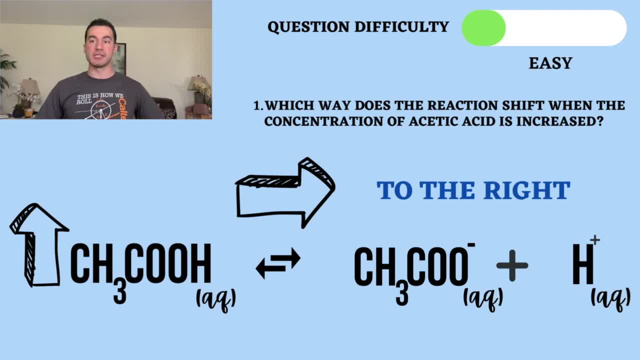 And that is exactly what ends up happening. I personally love doing Le Chatelier's principle questions with arrows. I usually put an up arrow and then an arrow going to the side that way. So, yes, it's going to end up going to the right as the products go up. 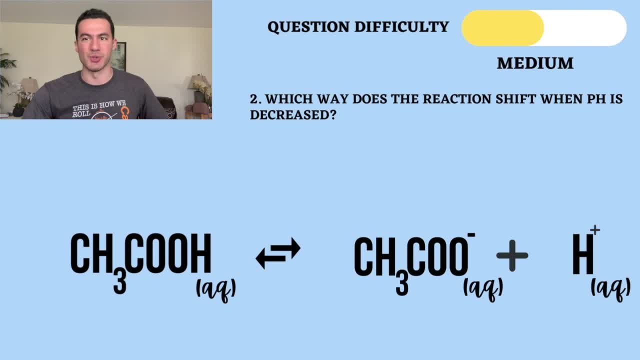 Hopefully that makes sense in question one, Question two. We're starting to get a little more difficult, And the reason why is because the way question two is presented is not all that straightforward. The question is saying: which way does the reaction shift when pH is decreased? 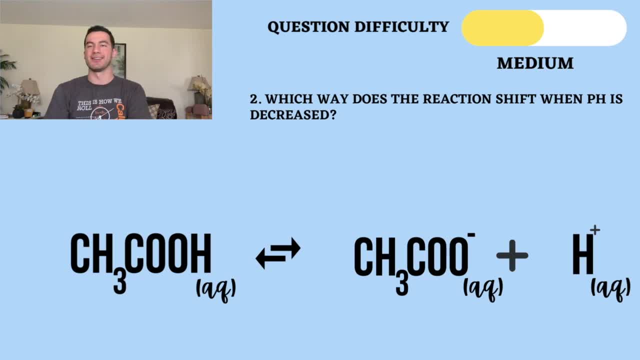 And some of you might be wondering: oh man, I don't know what happens when pH decreases? Well, when pH decreases, we know that pH is going to have more hydrogen ions, given that pH is equal to negative log of the hydrogen ion concentration. 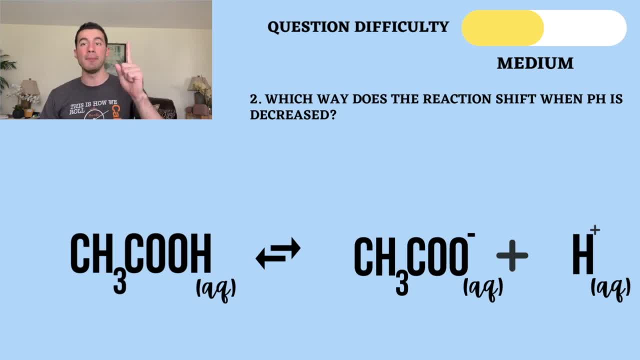 So, because of the negative log, as pH goes up, hydrogen ions go down. It has an inverse relationship. So when pH decreases, the amount of hydrogen ion concentration should increase as well. So as hydrogen ions increase, we're going to increase the products. 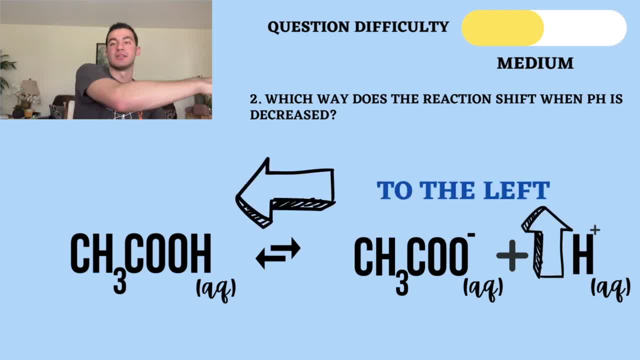 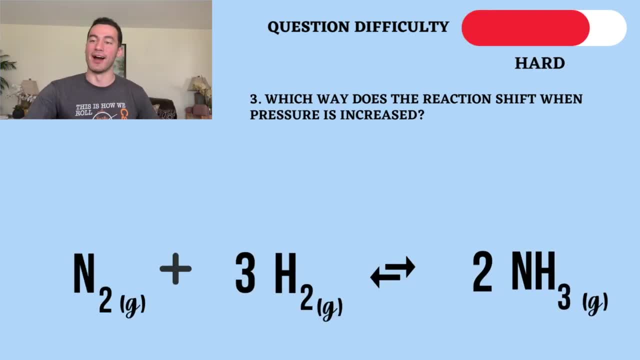 So we are going to favor the reactants. So it's going to form more acetic acid, aka shift to the left. That's exactly what we're going to get in this question. All right, So we're going on to question three. 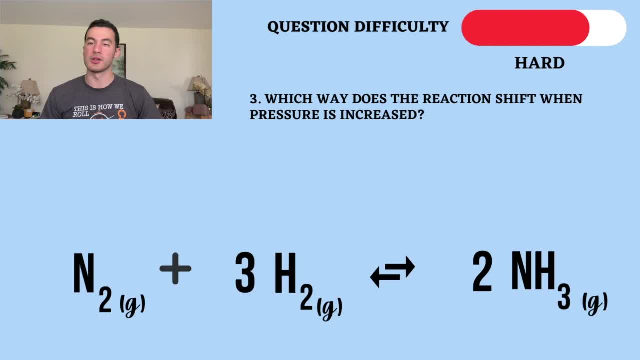 Which way does the reaction shift when pressure is increased? So note here that, as the questions get harder, what they're asking is a bit less direct than it was before, Because question one was asking what happens if you simply add more acetic acid. 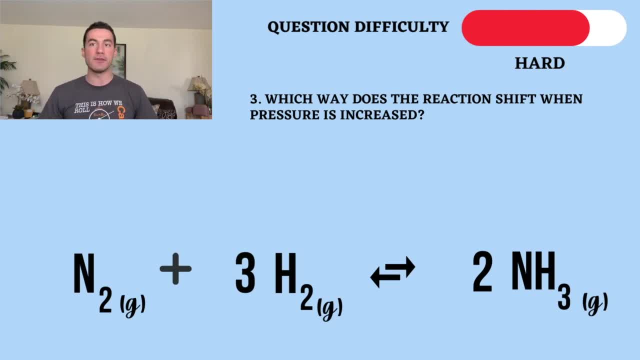 Question two was localizing. So he's saying: what happens if you add more hydrogen ions, but in a different language. Now question three is even more indirect. So we have to think of it this way: What happens when pressure is increased? 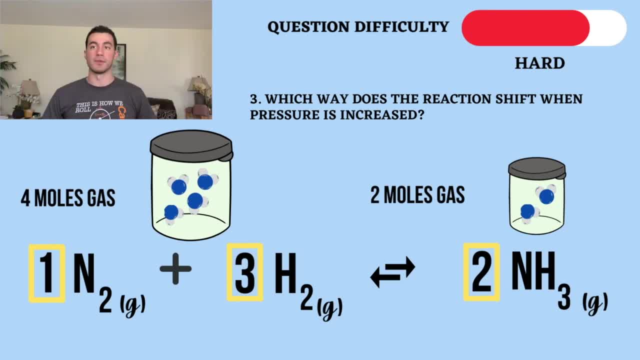 Well, when pressure is increased, volume ends up decreasing, So you end up having less space. And, in particular, I want to note that the last two questions they were about aqueous solutions, Whereas this question is dealing with the gas. 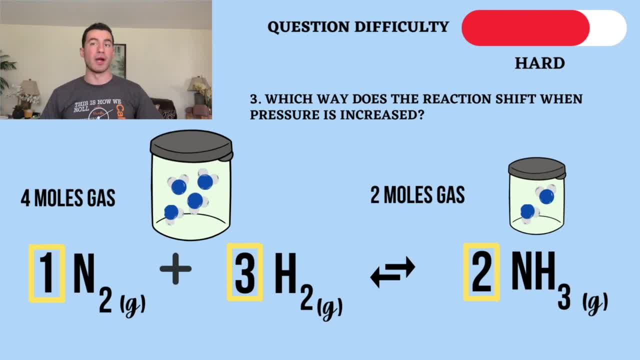 So gases they can be compressed into different volumes, Whereas liquids cannot, because liquids are incompressible. So when we increase pressure, that means we have more gas molecules in a smaller space, which is exactly what's going on in this scenario. 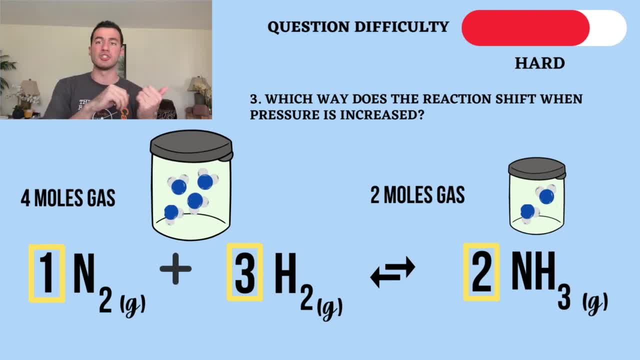 So, in order to solve this question and to understand which way the reaction is going to shift, we need to think of it this way, Because pressure means that you put gas molecules together. Imagine if I were to have a party at my house and 100 people were to come. 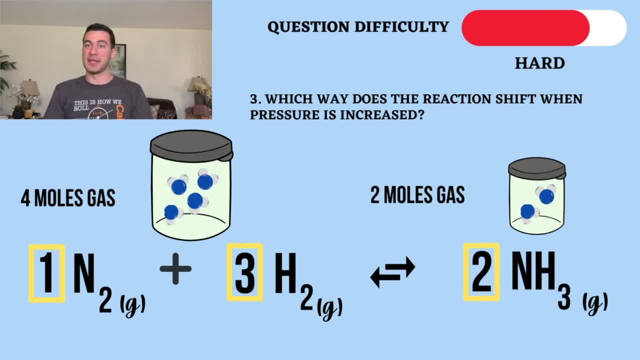 My house cannot fit 100 people in. It would not be too favorable. It would be a lot more suitable if 10 people came in And if my house were much smaller, it could be more suitable to a party, perhaps, of 10 people. 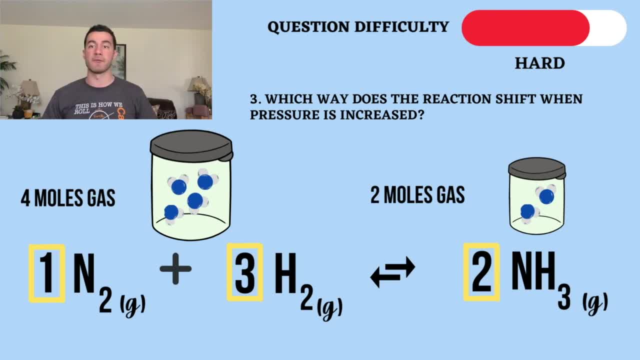 The same thing is going on when pressure increases. It prefers that there are less moles of gas within a space because it's able to fit them in, as explained by this little gas tank or pressure jar I have right here in these images down below. 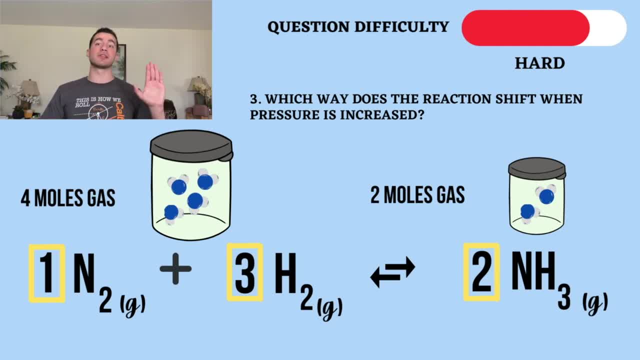 So in the first image we see that on the reactant side we have four moles of gas, We have one mole of nitrogen and we have three moles of hydrogen. And I put the yellow boxes around The coefficients Because in order to count moles, 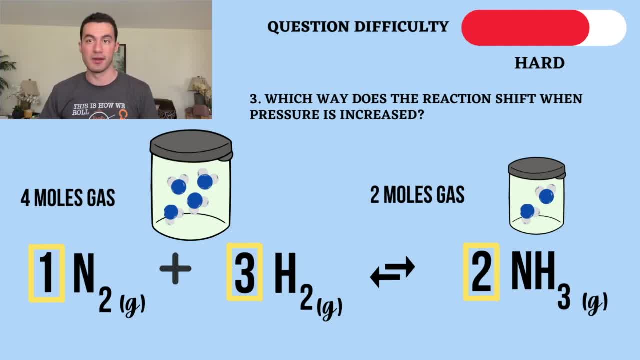 you're counting the coefficients of each reactant and each product, So you want to compare coefficients. You want to add up all the coefficients on the reactants, So one plus three makes four, And then all of the coefficients in the products. 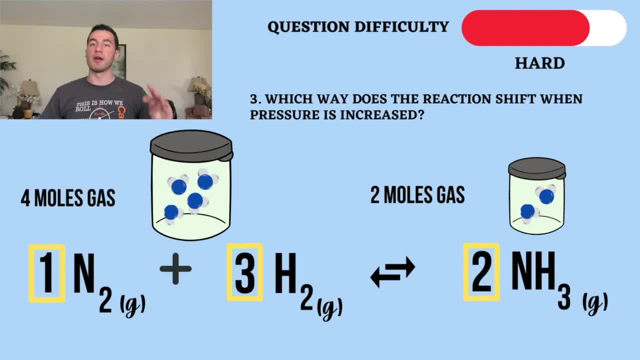 So we just have two, which still makes two. So we have four moles of gas in the reactants, two moles of gas in the product. The equilibrium is going to end up shifting right, because higher pressures favor lower moles of gases.